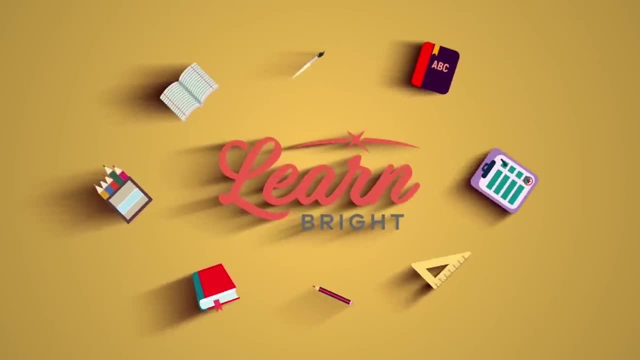 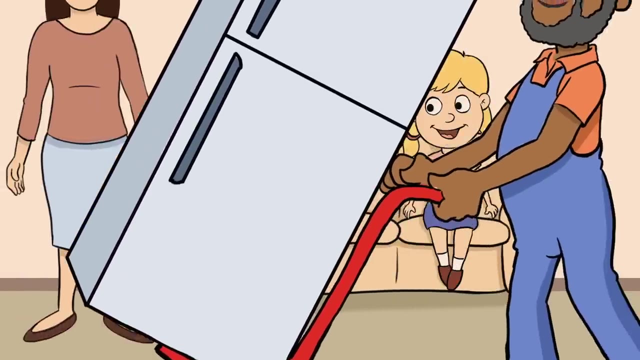 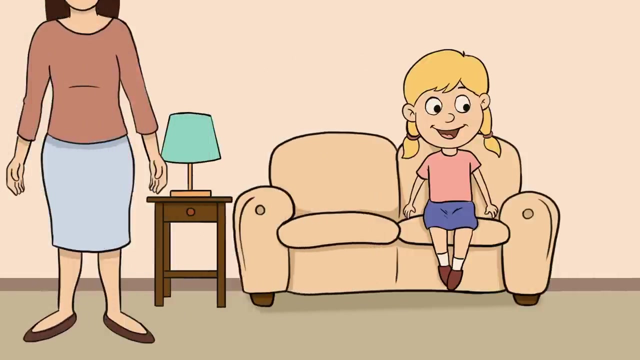 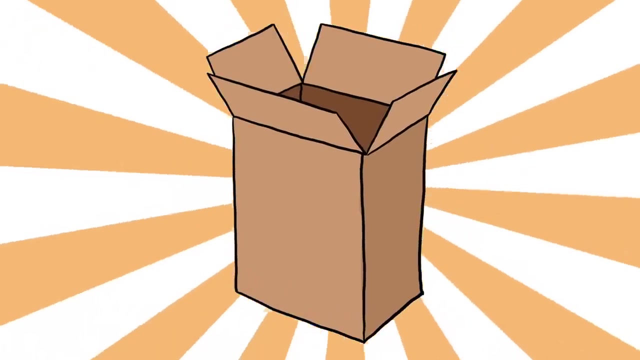 Oh, wow. Not so long ago, when I was your age, my mom bought a new refrigerator. I remember how excited she was. I didn't care much about the fridge until I saw the biggest, most amazing box I had ever seen in my life. It was three times as big as I was and seemed like it took up half 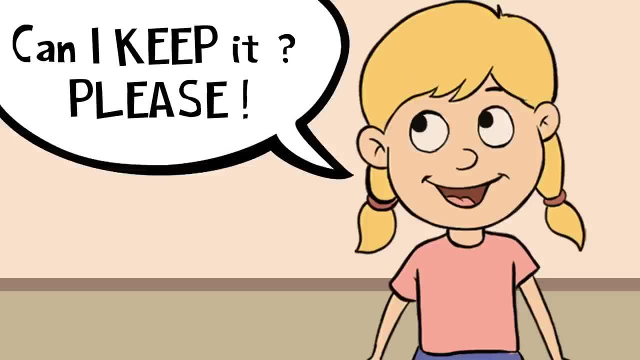 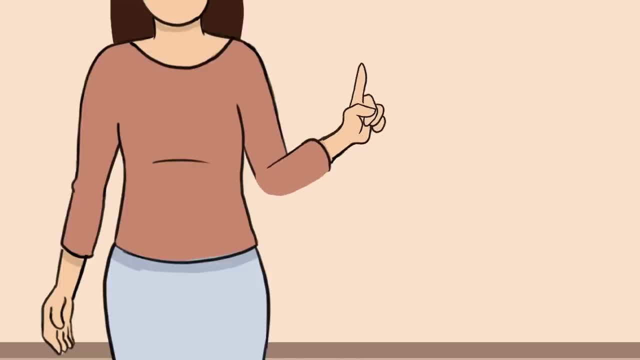 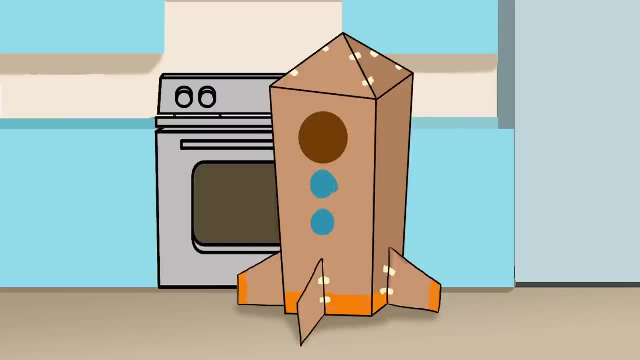 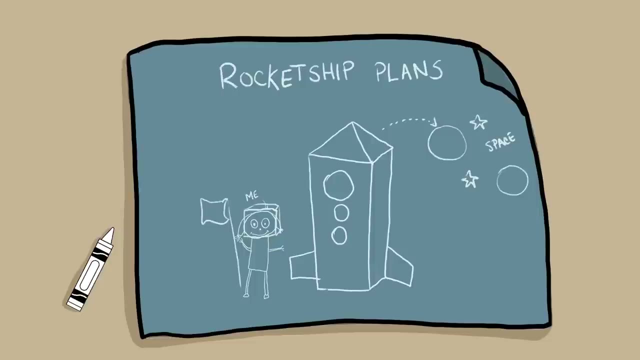 the kitchen. I shouted across the room to my mom: can I keep it please? After some convincing, she agreed on one condition: It had to stay outside. That's perfect, I said excitedly, because rocket ships do not belong in kitchens. I spent two weeks building the perfect rocket ship. 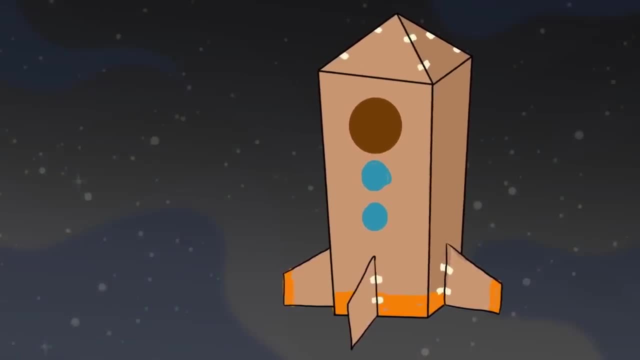 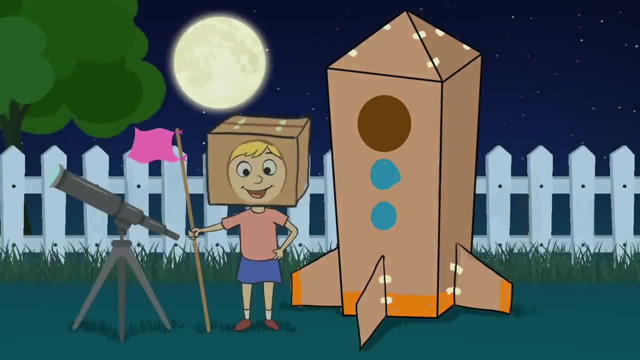 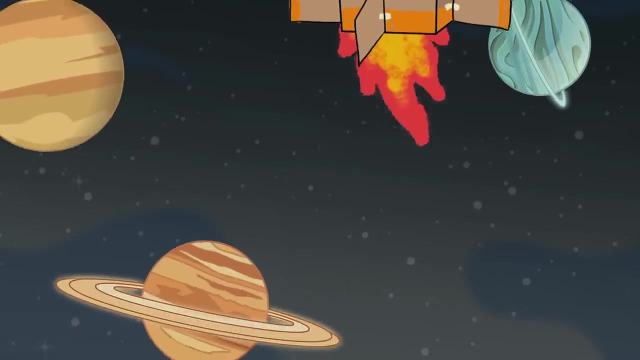 with orange and blue paint and windows to see the stars At night. I had so much fun that summer learning how to use a telescope, going on pretend trips to space, looking at stars and imagining what it would be like to visit all the planets in our 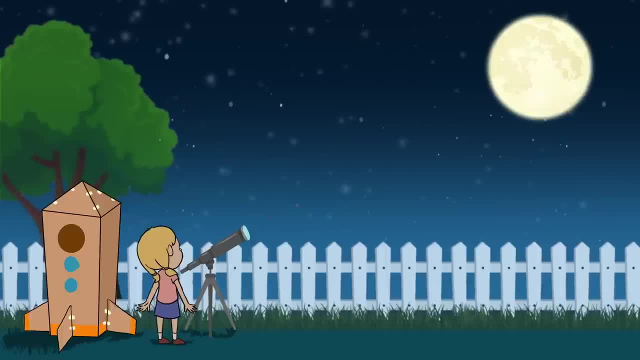 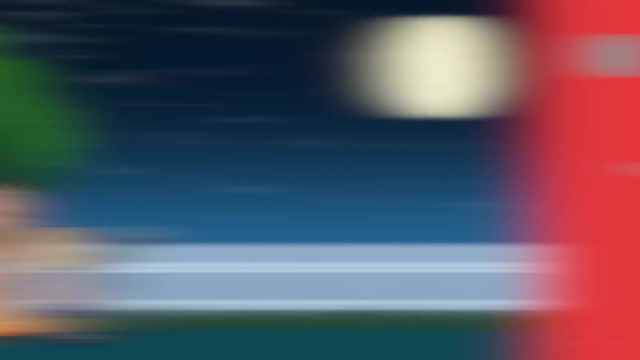 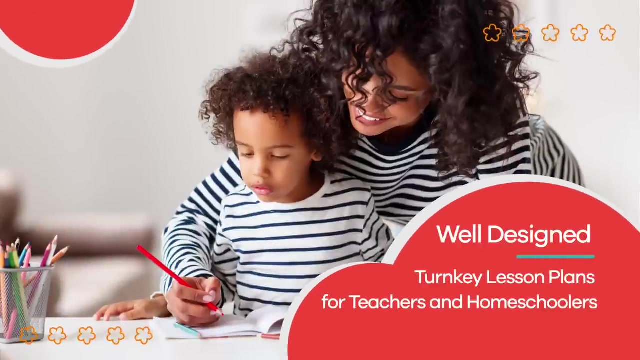 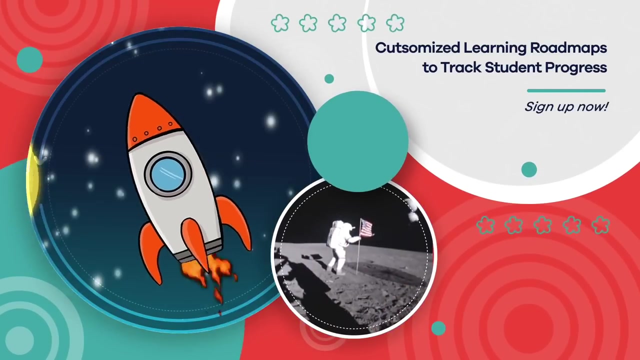 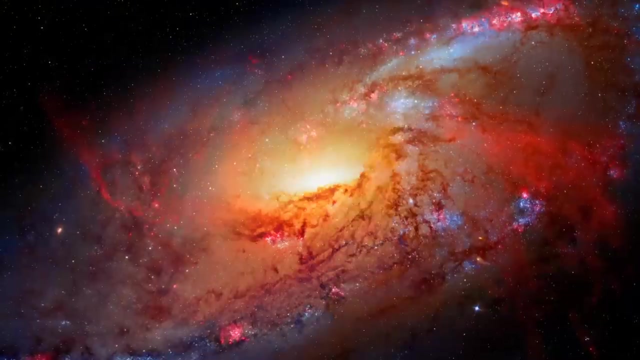 solar system That summer. even though my trips to space were totally pretend, the moon and stars and planets we saw with our telescope were all very real. They are all part, part of a larger planetary system called a galaxy. A galaxy, by definition, is a system of millions or even billions of stars. 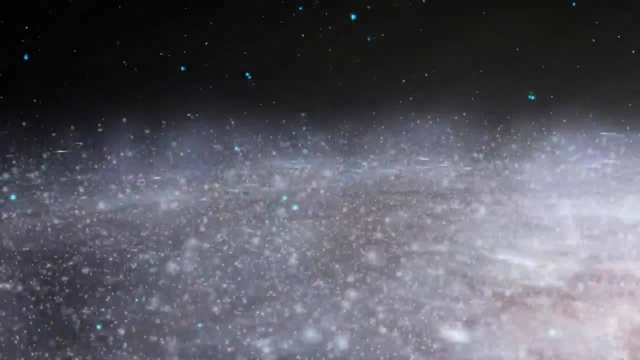 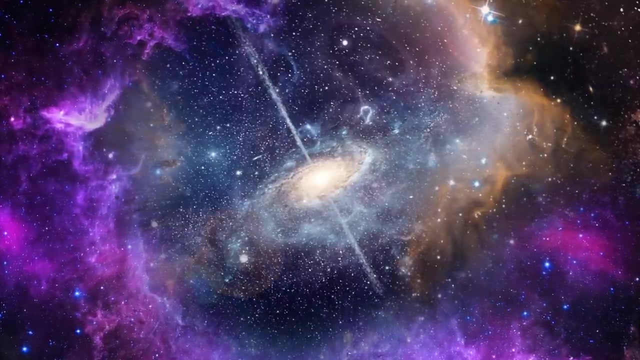 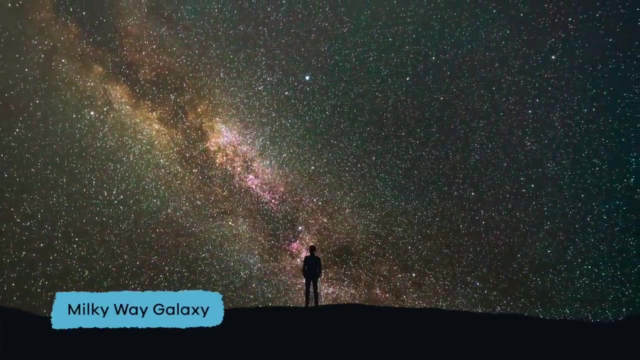 The galaxy is a sum of stars, dust and gas that is all held together by gravity, which keeps it all in place. Galaxies are enormous and our universe is made up of billions of them. The name of our galaxy is the Milky Way Galaxy. It gets its name because all those white stars look like a giant spilled glass of milk. 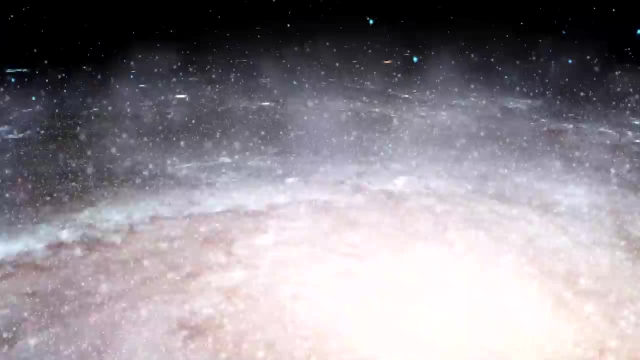 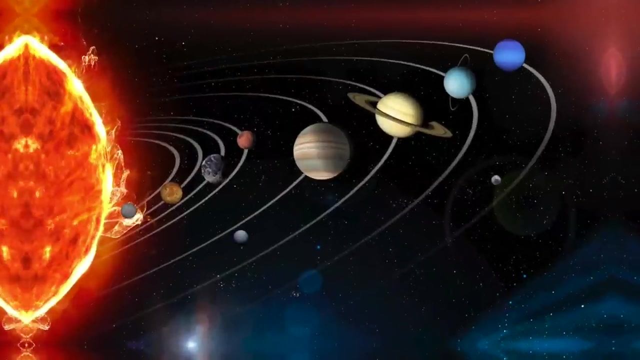 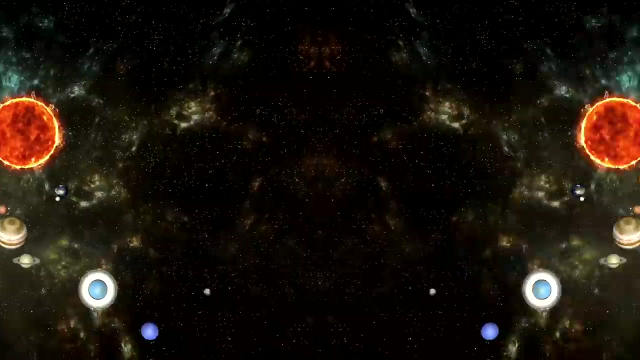 Let's talk about what's inside the Milky Way. And no, it's not king caramel, but that would be super awesome. This is a picture of our solar system. Our solar system is you-nor-mous. That's not actually a word, but it is very, very big. 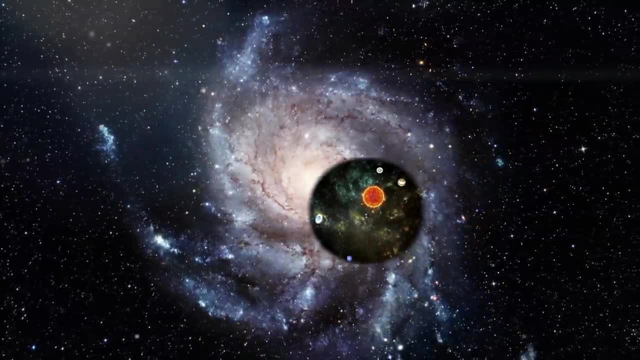 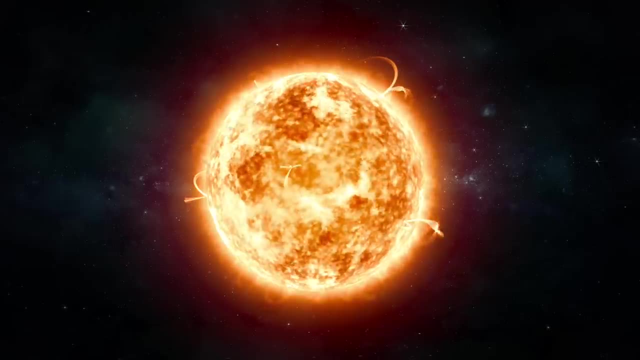 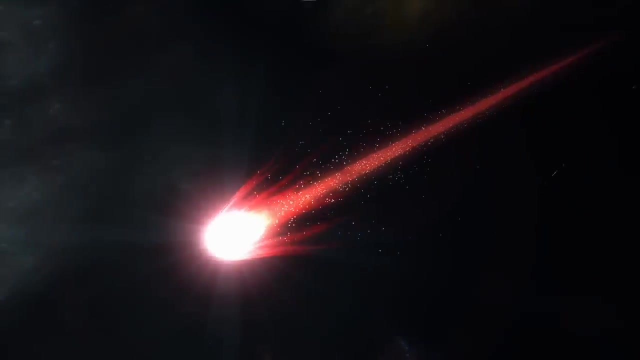 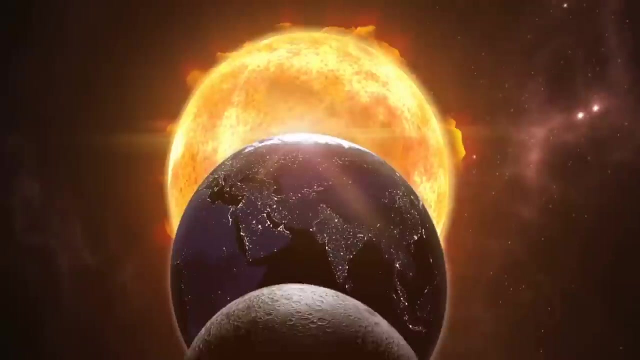 And our solar system fits inside the Milky Way galaxy, which gives you an idea just how massive our galaxy really is. The Moon, the Sun, eight planets, including Earth, space rocks and other cool things, are all part of that solar system, But in this video we are going to focus on our eight planets. 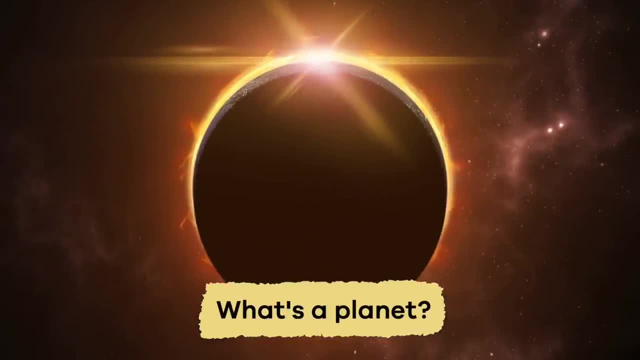 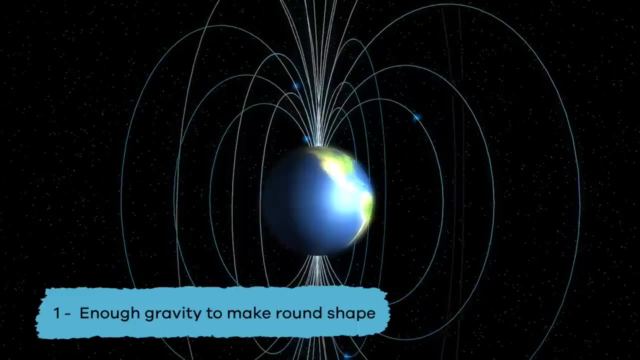 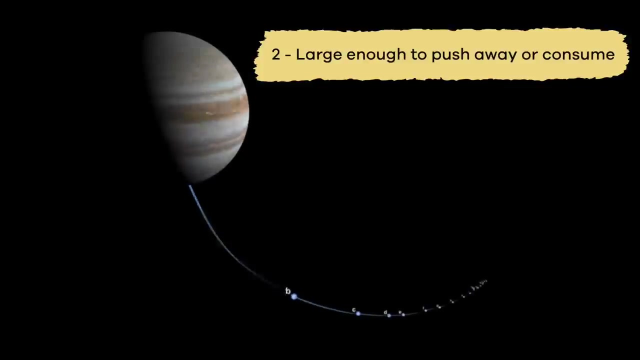 So what's a planet? To be considered a planet requires three things. One, it is a large object with enough gravity to pull itself into a round shape. Two, It must be big enough to push away or consume other objects in its path. 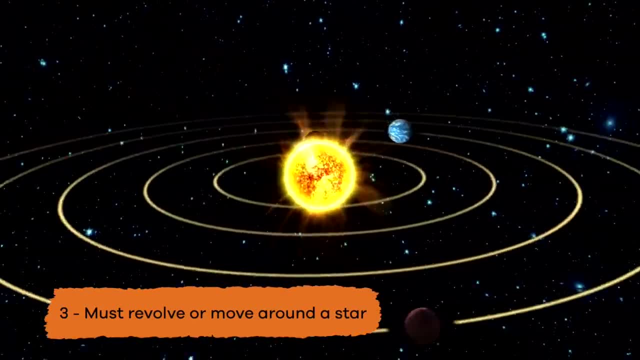 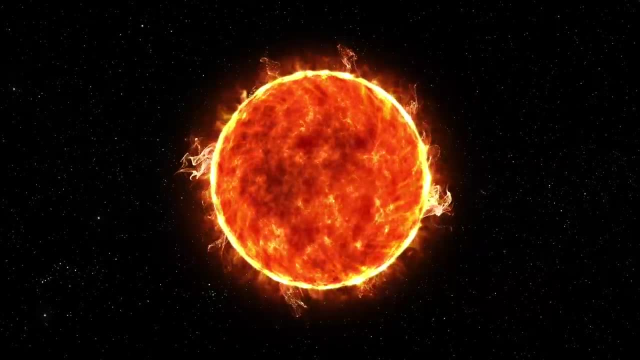 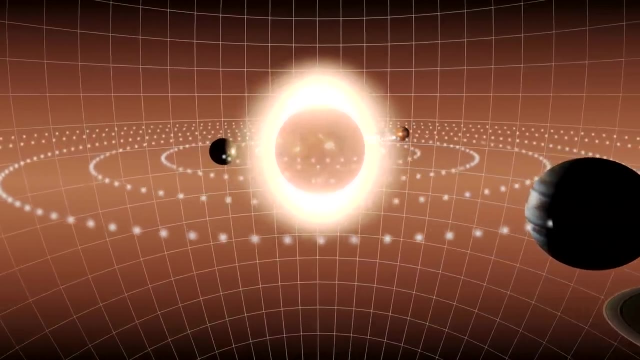 And three: It must revolve or move around a star. In our solar system. that star is the Sun. Yep, the Sun is a massive star, And the eight planets in our solar system all revolve or move around that star. One thing that makes each of the planets unique is that they all revolve around a star. 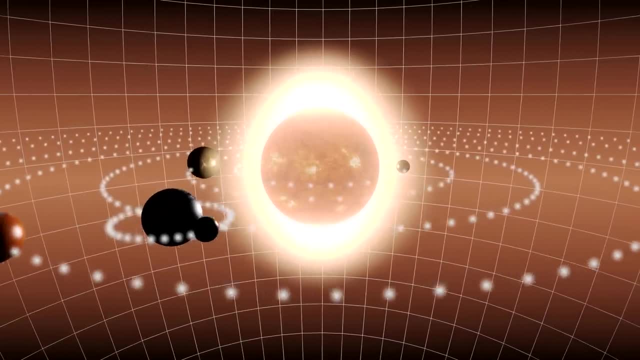 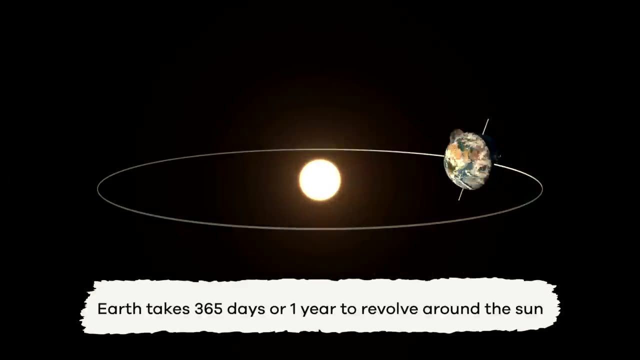 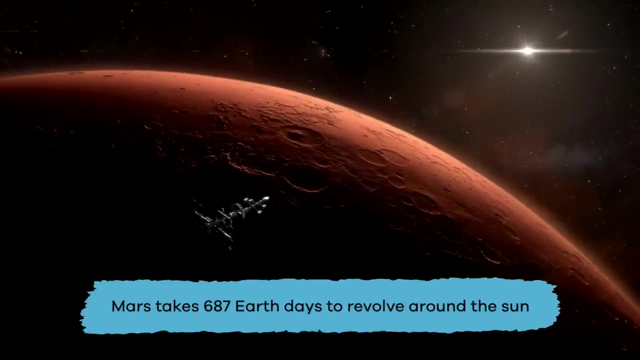 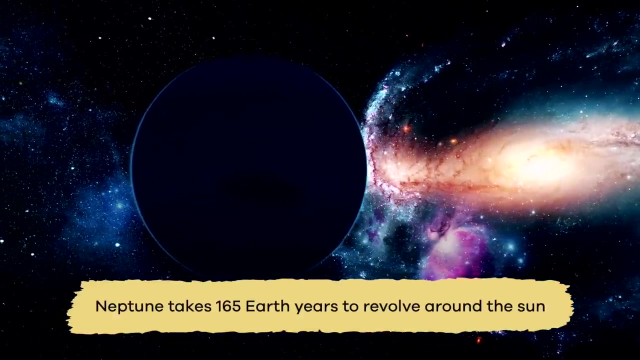 For example, it takes 365 days or one year for the Earth to revolve just one time around the Sun. On Mars it takes almost twice that long, And on Neptune it takes 165 Earth years for it to move around the Sun once. 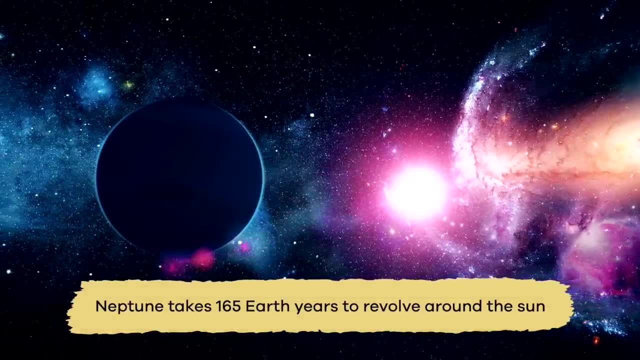 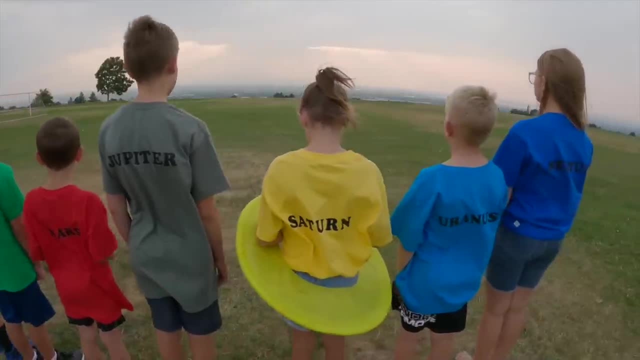 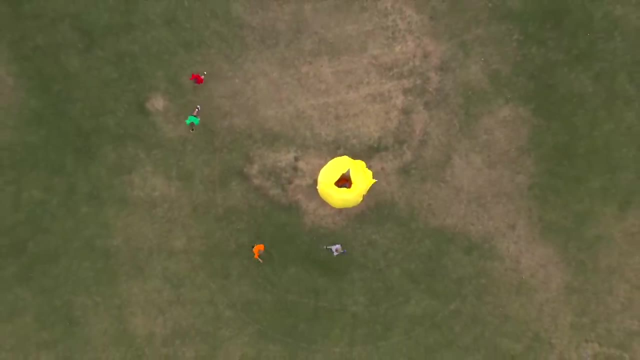 But is Neptune just super slow? No, it's not. Or is there another reason it takes Neptune so long to orbit the Sun? Take a look at these eight kids standing around a big yellow ball. The ball represents the Sun and the kids represent each of the planets. 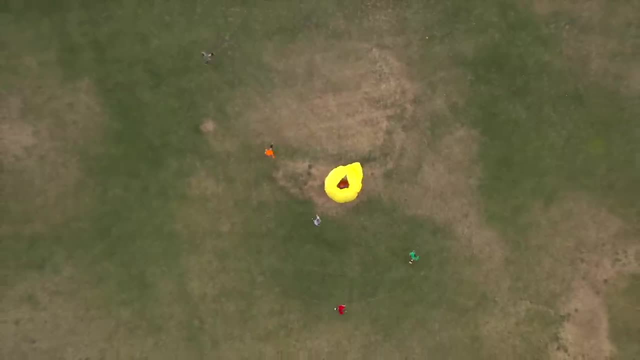 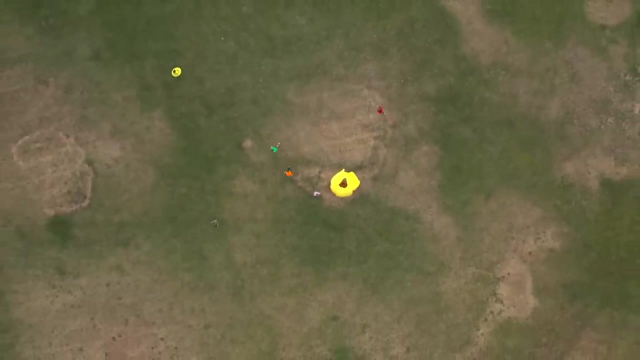 Now watch what happens when they start to move or revolve around the Sun. What do you notice is happening? What do you notice is happening? What do you notice is happening? Some of the kids are able to move around the ball quicker than other kids. 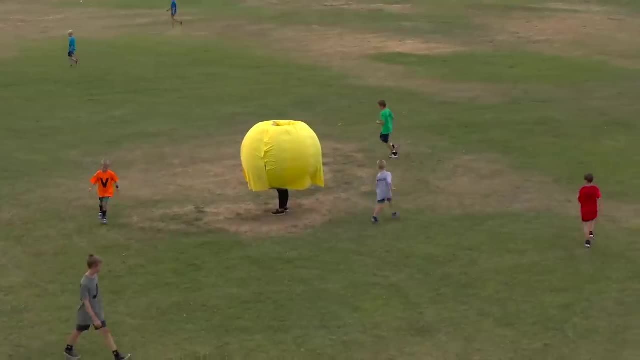 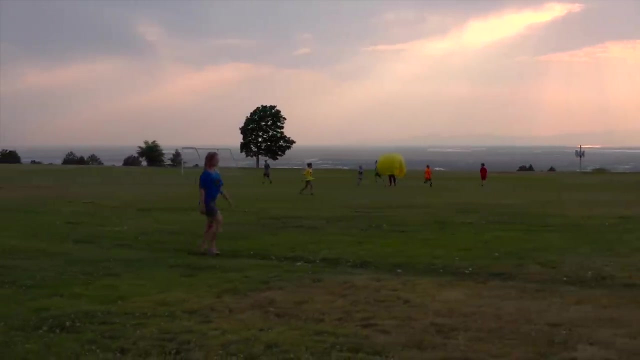 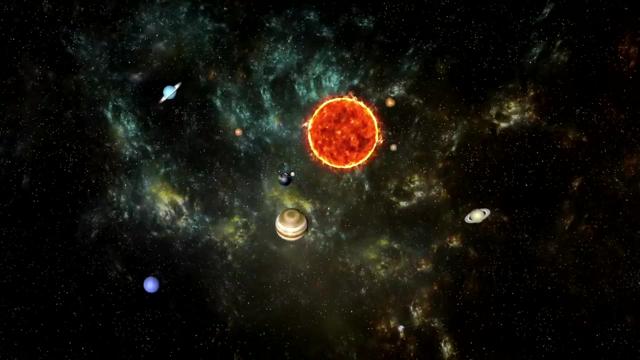 That's because they are closer to the ball, so they have less distance to travel. The kids are also different sizes and some are faster than others. Just like the kids and the yellow ball, the planets are also different distances from the Sun. 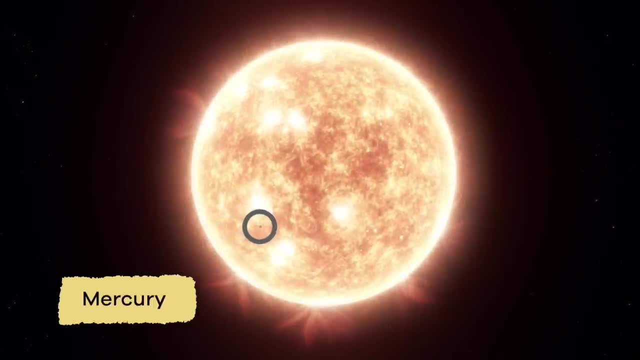 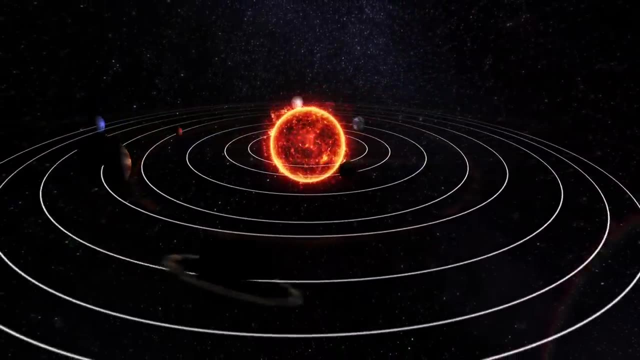 The planets that are closest to the Sun have the shortest distance to move, while the planets that are farthest away from the Sun have a longer distance to go, And, just like with the kids, the size and mass of each planet also affects their speed. 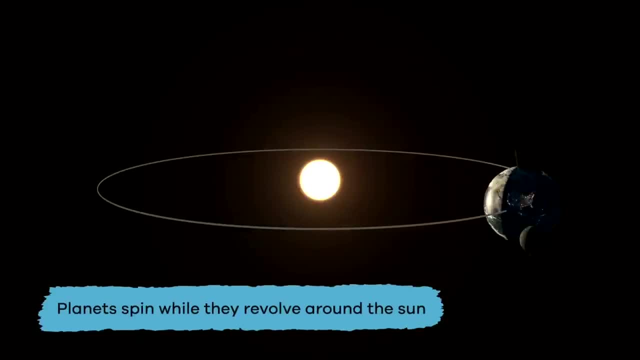 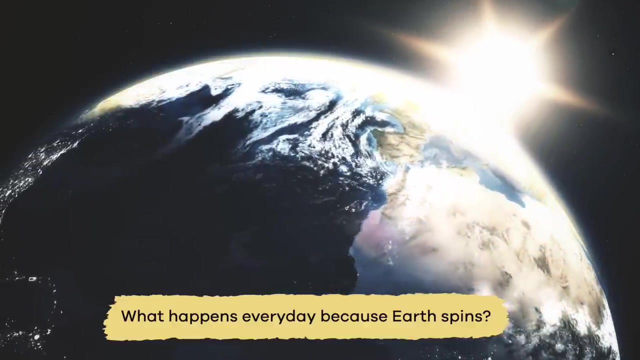 Cool planet fact: Not only do the planets revolve around the Sun, but they also spin while they are revolving. Can you think of something that happens every day on Earth? because Earth spins? No, Have you ever wondered where the Sun goes each night? 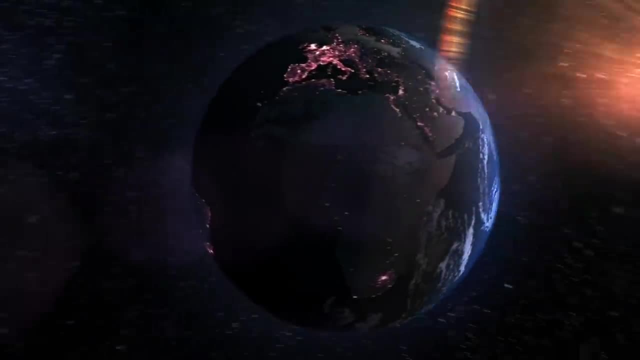 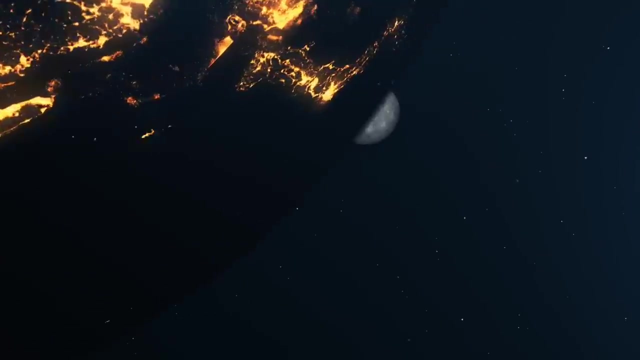 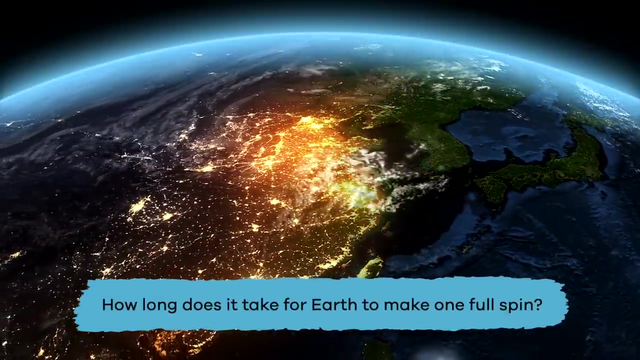 It doesn't actually go anywhere. It's the Earth that moves, And when it's daytime on one side of the planet, it's nighttime on the other. Guess how long it takes Earth to make one full spin. Did you say 24 hours? 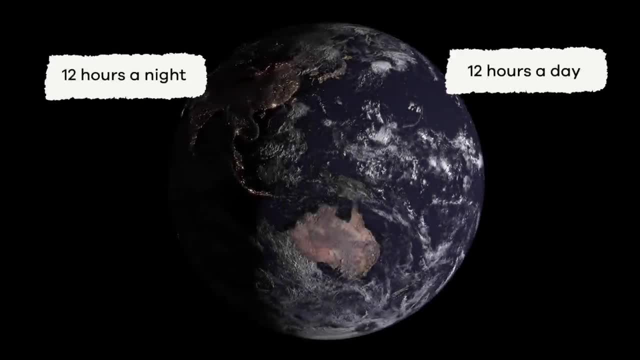 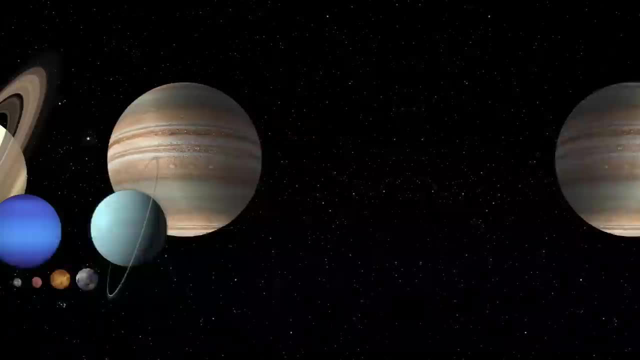 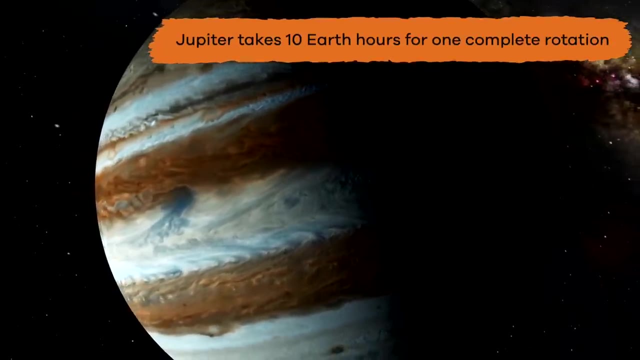 You're right: 12 hours during the day and 12 hours during the night. And just like the planets don't revolve at the same speed, they don't spin at the same speed either. On Jupiter, it takes less than 10 Earth hours to make one full spin. 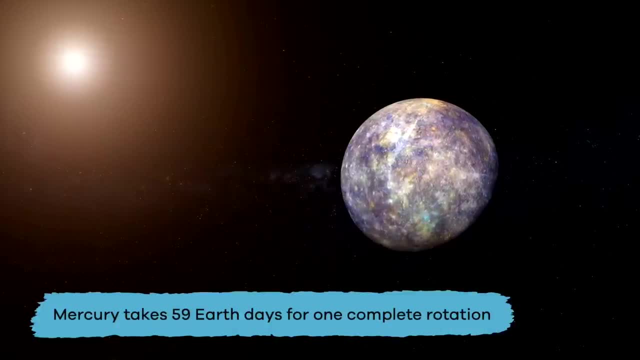 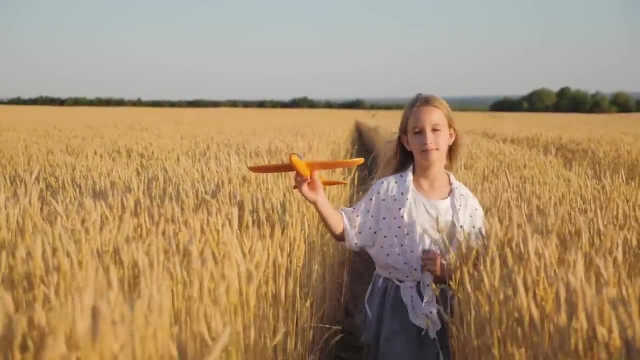 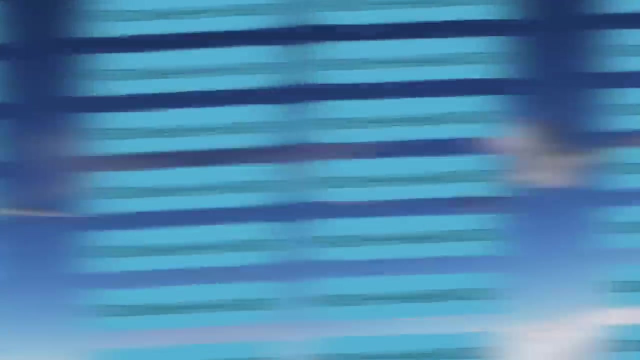 But on Mercury it takes 59 Earth days. By the way, have you ever wondered why you can't feel the Earth spinning? If you've ever flown on an airplane, that plane was probably traveling at about 500 miles per hour. That's about five times faster than your car goes. 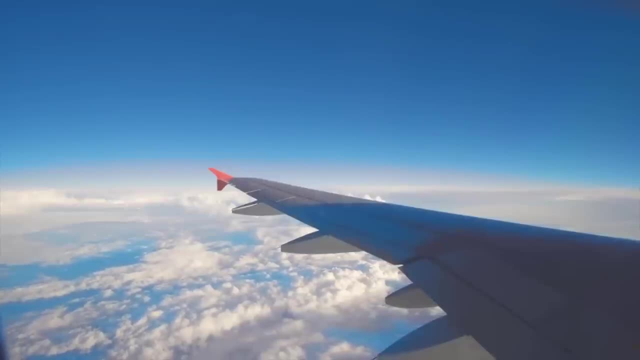 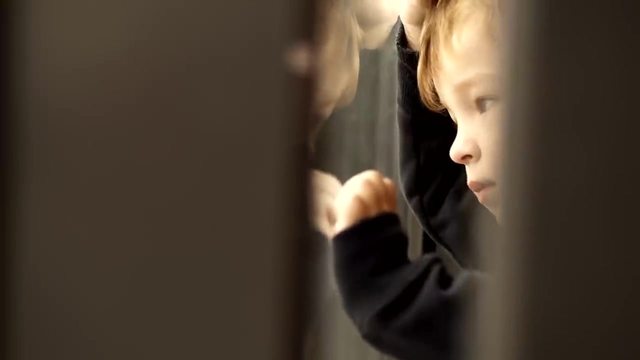 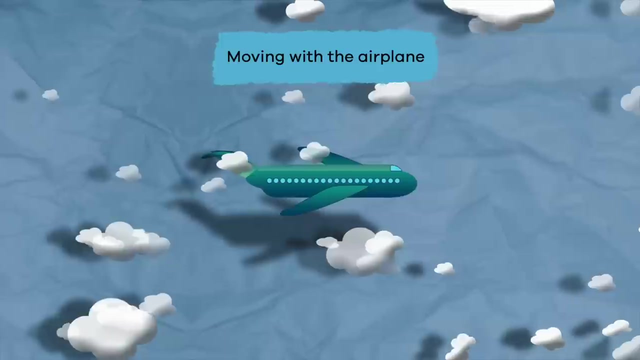 That's pretty fast, But when you're in an airplane it doesn't feel like it's moving at all. In fact, on longer trips you might even wish it moved faster. The reason you don't feel like you're moving on an airplane is because you are moving with 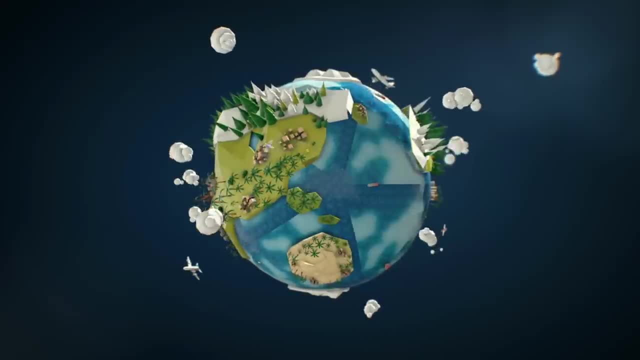 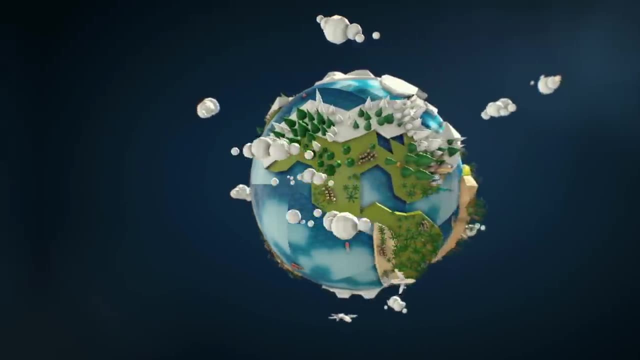 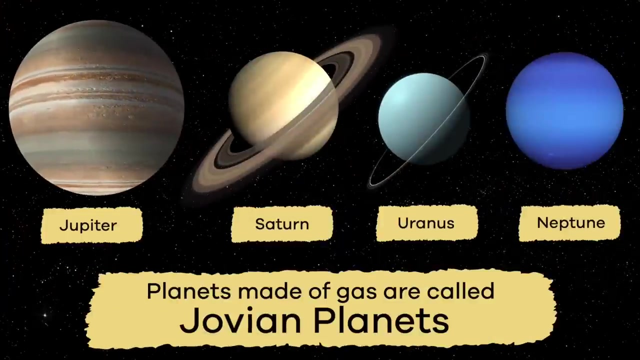 the airplane. Since we're on Earth and the Earth is spinning, we spin with it and don't even notice it. Cool planet fact: Some of the planets are made of rock, while others are made of gases, which means those planets are not completely solid. 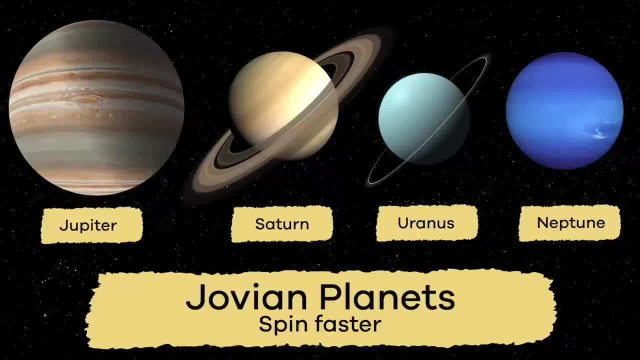 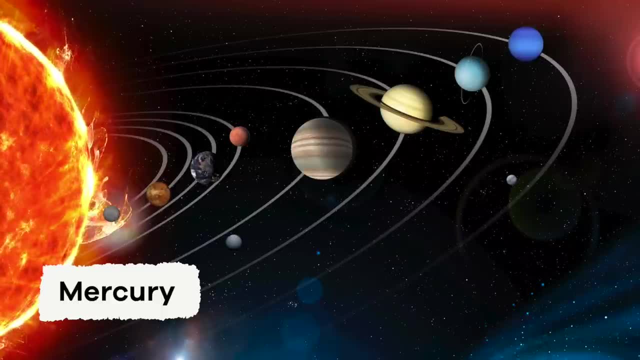 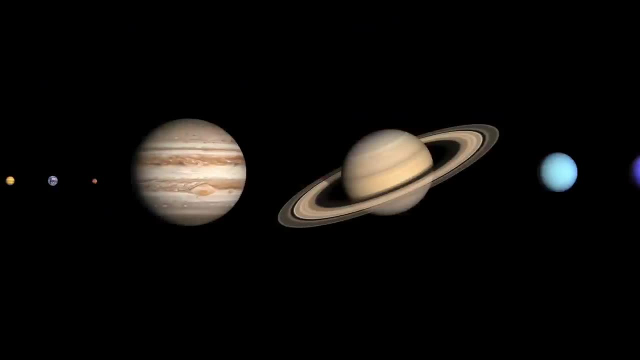 The planets made of gas spin quicker than the planets made of rock. Let's take a closer look at each of our planets. Our journey begins with Mercury. Mercury is the closest planet to the Sun. It is also the smallest of the eight planets. 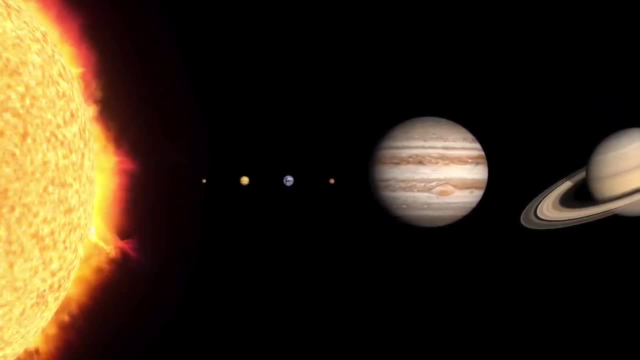 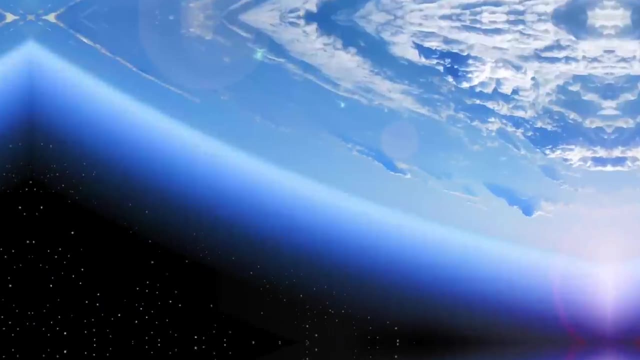 It's about the same size as the Moon and has very little atmosphere. Atmosphere is like a see-through shield that protects planets from space rocks and other debris. So if there isn't much atmosphere, then Mercury is the closest planet to the Sun. 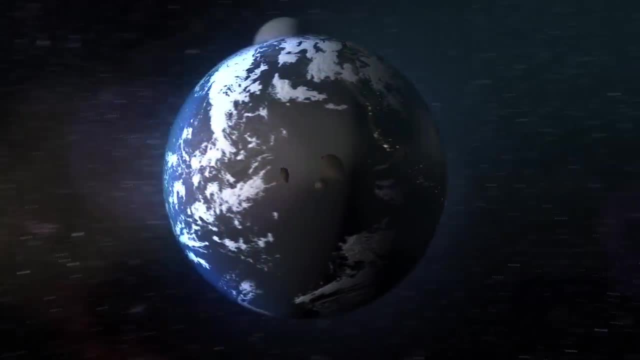 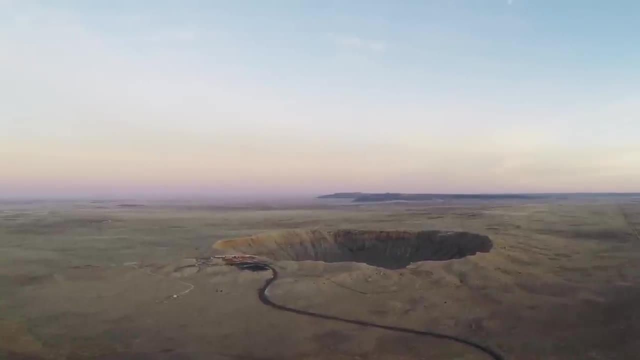 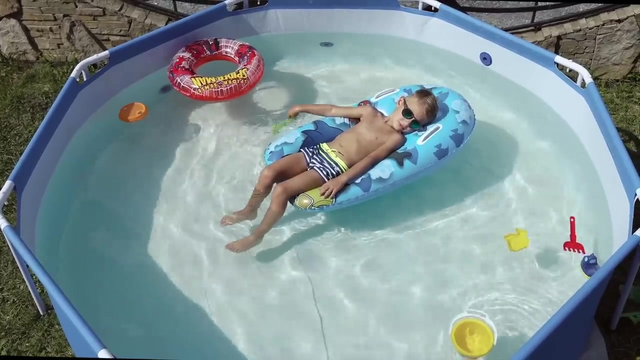 Mercury is the closest planet to the Sun. Mercury is the closest planet to the Sun. When there isn't much atmosphere, those rocks can end up hitting the planet, creating giant holes or craters. Mercury is also very, very hot. Think of 100 degrees Fahrenheit in summer. 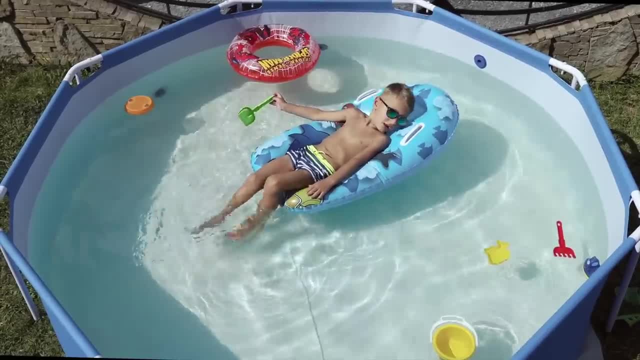 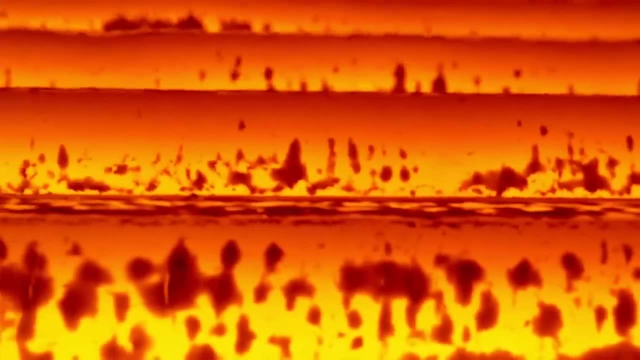 How does your body feel? How long can you stay out in that heat? How long would a popsicle last before it melts? Now imagine if it was eight times hotter than that. How long would a popsicle last before it melts? How long would a popsicle last before it melts? 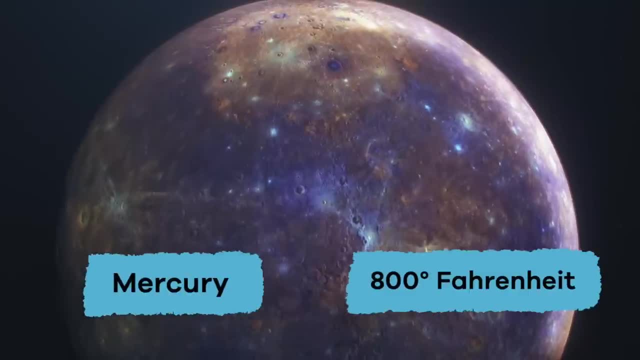 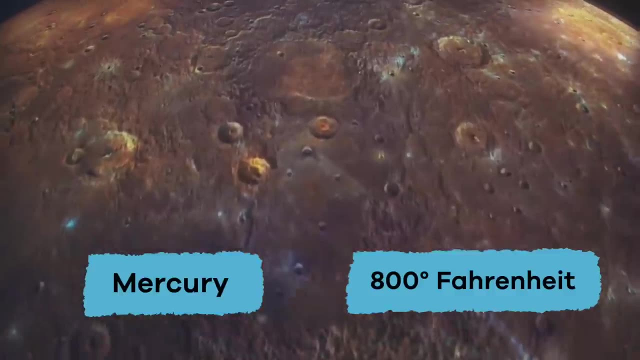 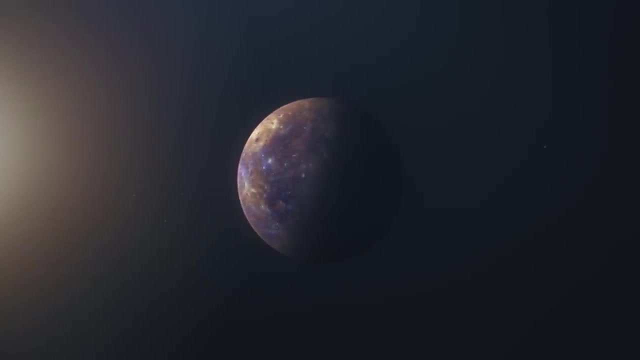 Let me know in the comments below. That's the temperature on Mercury during the day. If you've ever wondered why people don't live on other planets, heat is a big reason for mercury. However, Mercury is not the hottest planet in our solar system. 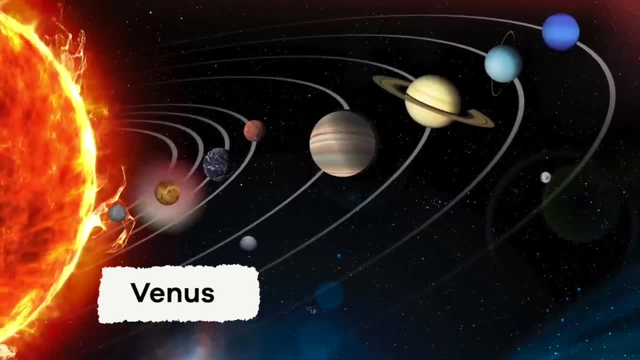 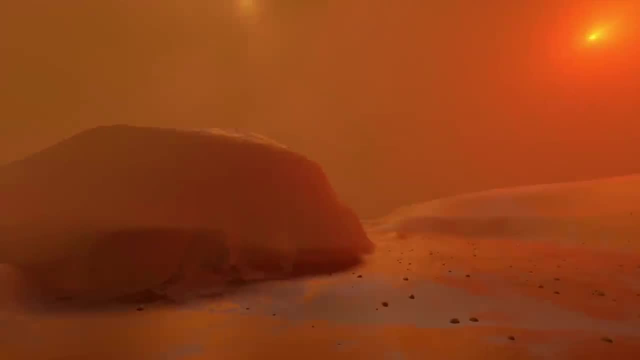 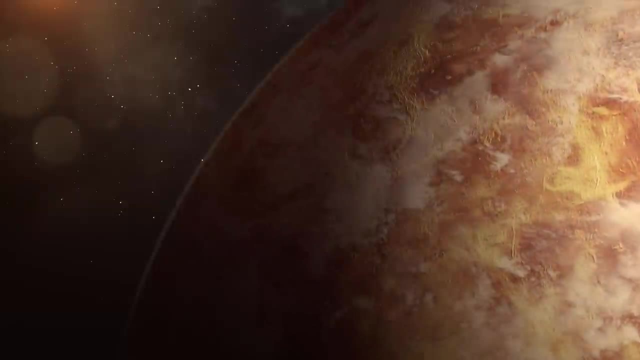 Venus is. Even though Venus is not the closest planet to the Sun, it is the hottest Mercury, which has a thin atmosphere. the atmosphere on Venus is very thick. Its atmosphere traps heat from the sun, so the planet gets extremely hot. Venus is about 900 degrees. 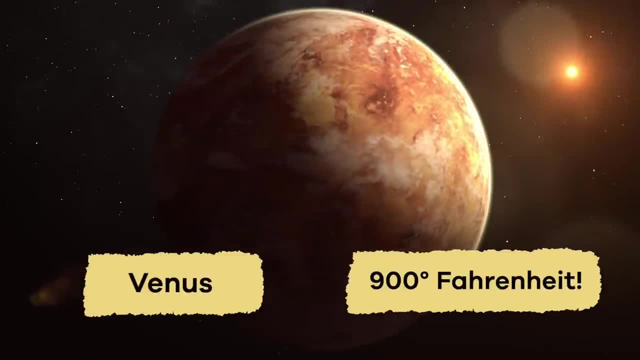 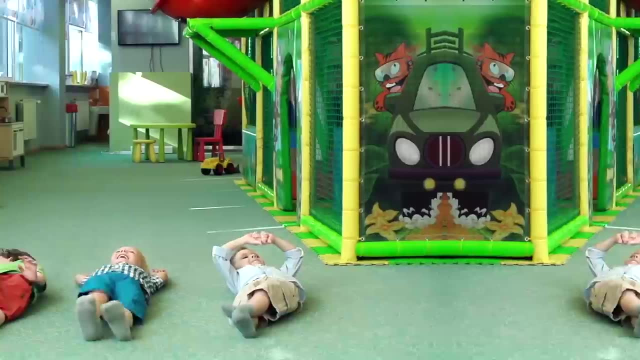 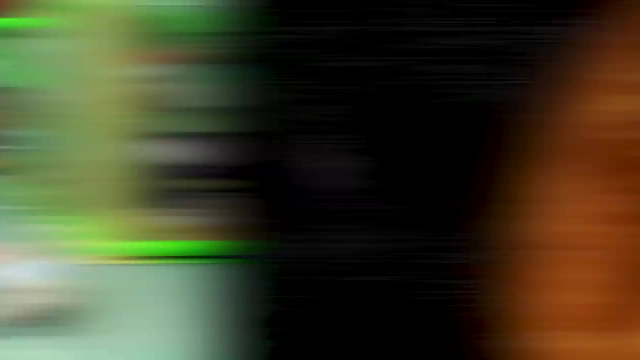 Fahrenheit, making it the hottest planet of them all. But that's not the only thing that makes Venus different from the other planets. Do you know any kids at your school that have to do the opposite of what every other kid is doing? Well, that's Venus. Venus spins. 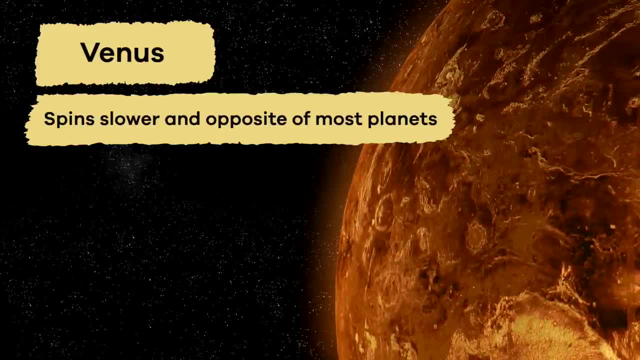 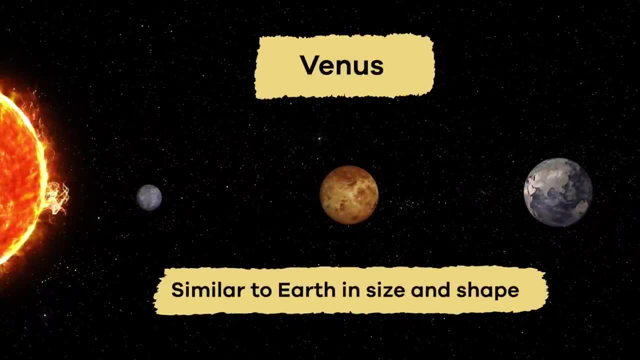 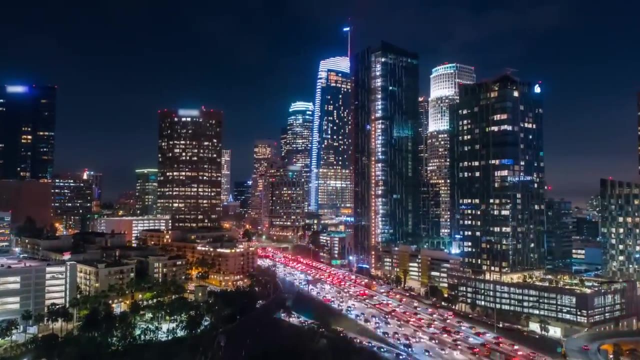 slowly and in the opposite direction of most planets. Even though Venus is a lot hotter than Earth, it is similar to Earth in size and shape. Speaking of Earth, Earth is where we live. It's the only planet where people live. Have you ever wondered why? Well, it's. 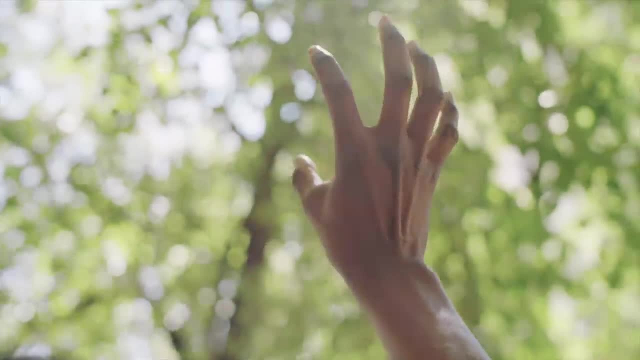 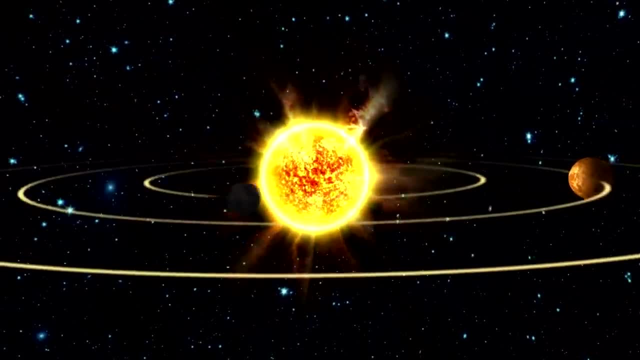 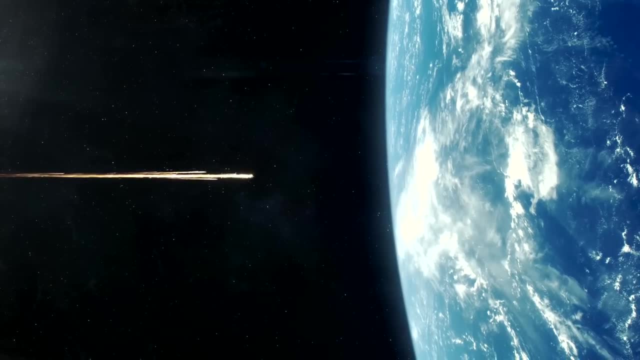 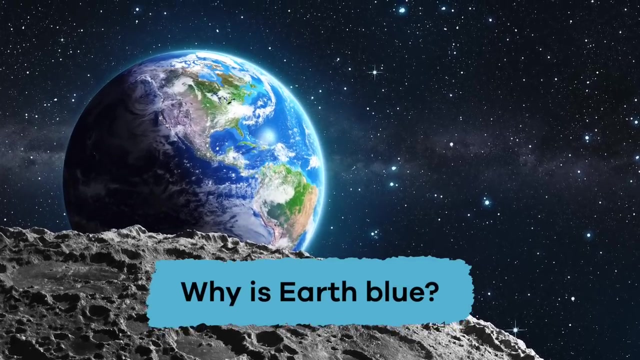 for life to exist here. Unlike Venus and Mercury and the other planets, Earth's atmosphere keeps us at just the right temperature and protects us from things in Space. Speaking of space, this is a picture of Earth from space. Can you guess why it's mostly blue? 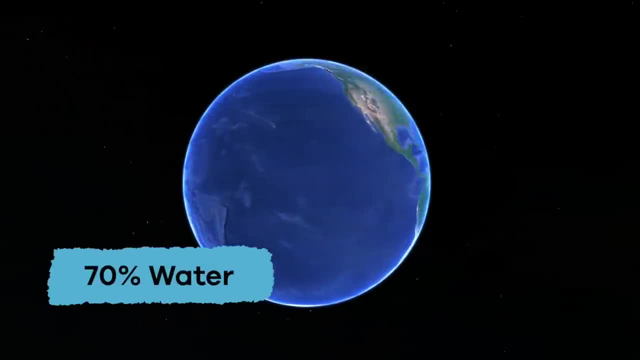 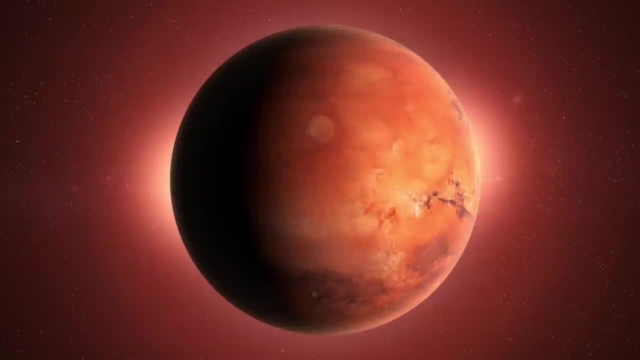 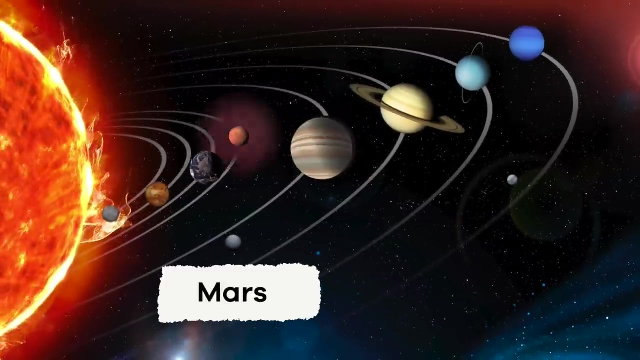 That's because 70% of Earth is made of water. Unlike Earth, our next planet has very little water on it, and what water it does have is frozen. Mars has the nickname Red Planet. Can you see why It gets that name from its rust-colored soil? 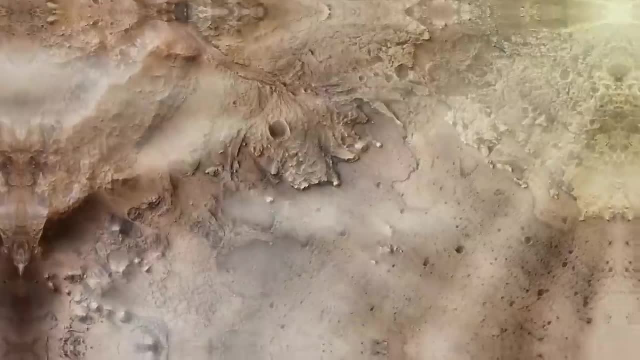 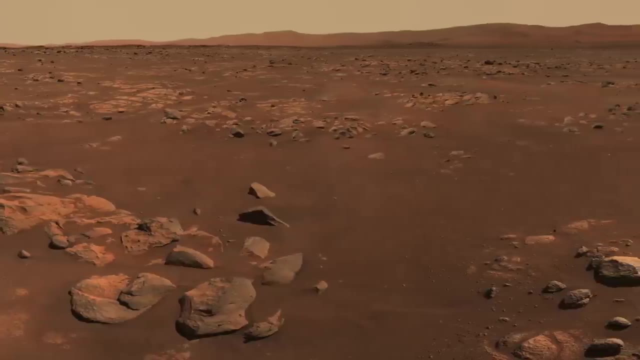 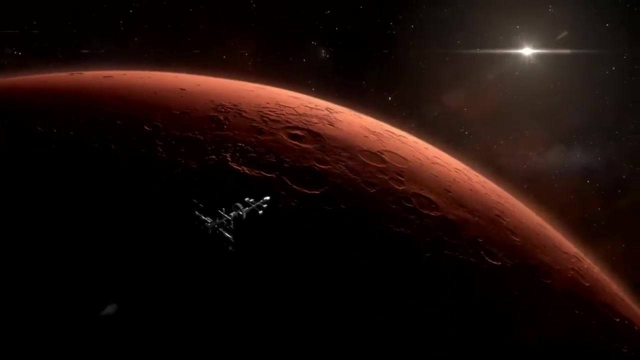 Mars is about half the size of Earth. Volcanoes, impacts from space, debris, wind and other things have all changed the surface of Mars over time. Several orbiters or space shuttles have flown by and around Mars and rovers. 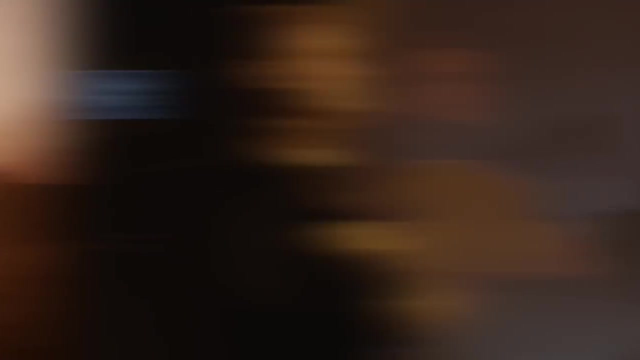 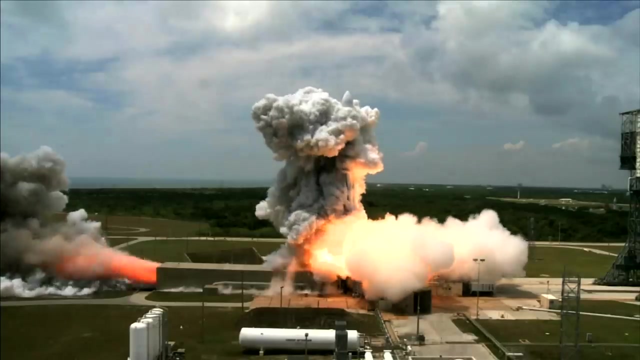 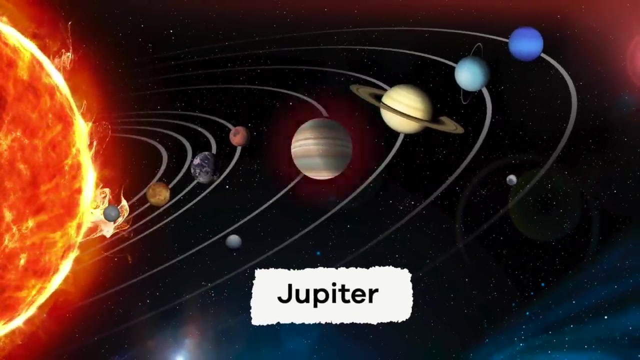 have even landed on its surface. If people were to ever live on another planet, Mars might be the most similar to Earth. In fact, some scientists are even making plans to land on Mars. Jupiter is the largest planet in our solar system. It's so big that if you took all the other planets, 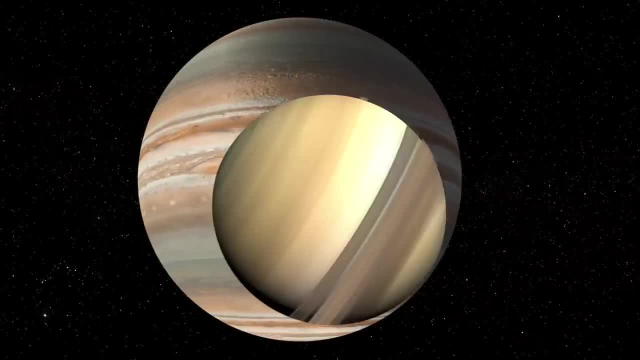 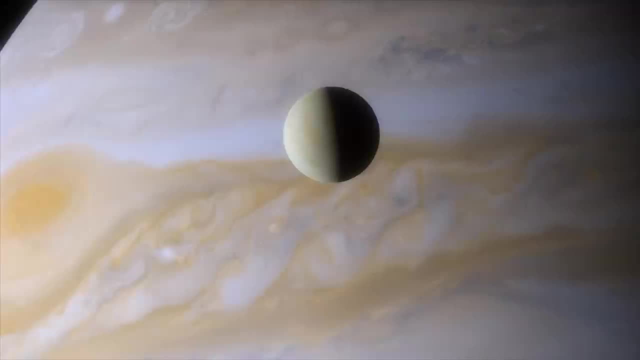 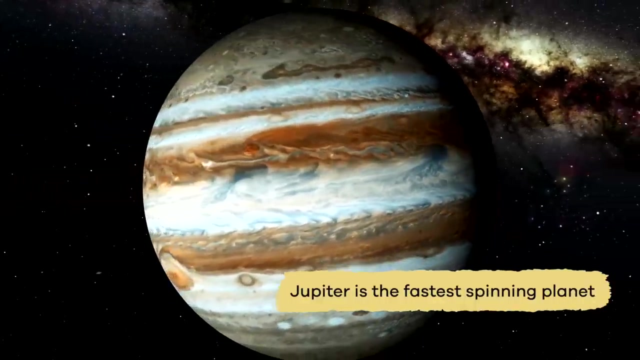 and squished them together, Jupiter would still be over two times bigger. Not only is Jupiter the biggest planet, but it is also the fastest-spinning planet in our solar system. Let's move on to Saturn. Saturn is the largest planet in the world. 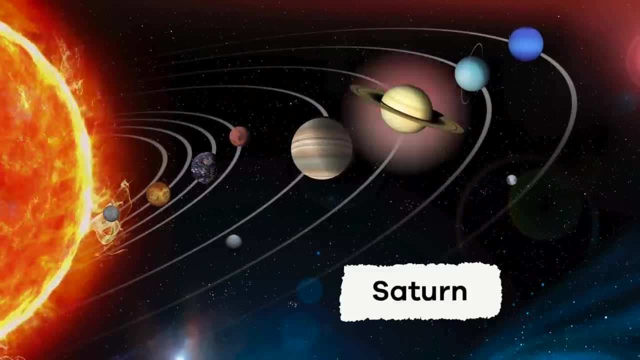 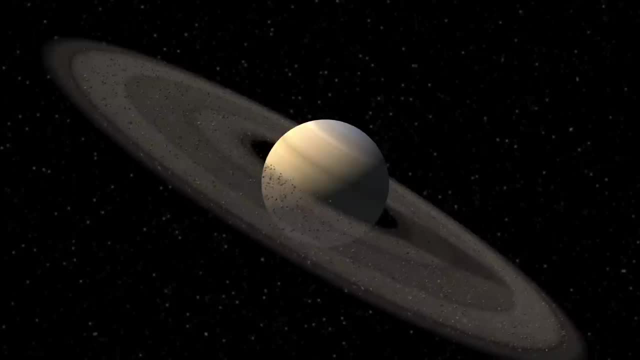 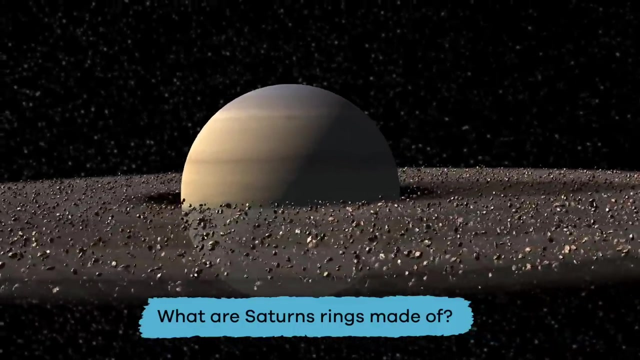 It's the largest planet in the world. Can you guess what makes this planet unique? Those rings are pretty cool, huh? Do you know what they're made of? We'll give you a hint: It's not gold. Scientists think that Saturn's rings are made up of bits. 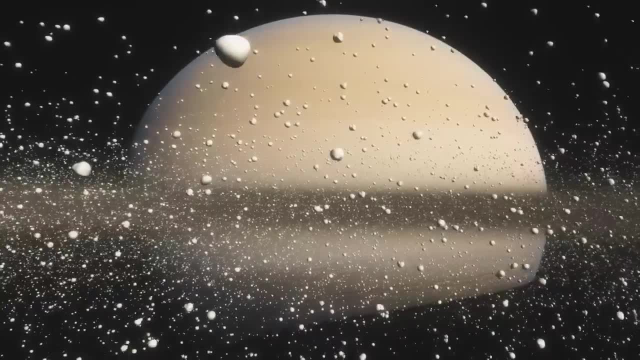 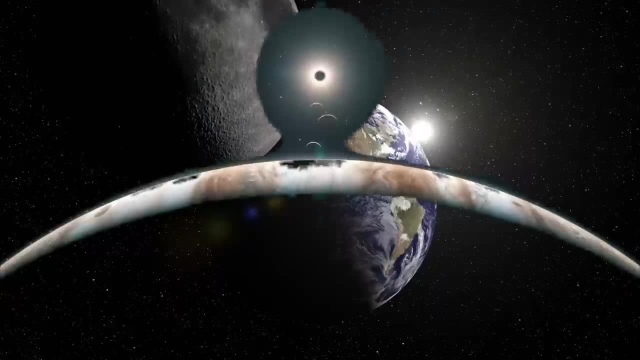 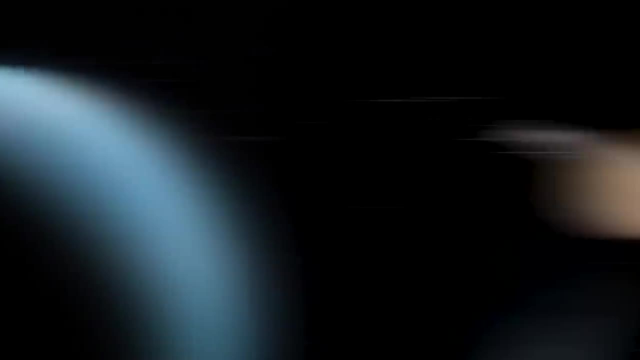 of space, rock and debris left over from moons. Hold on, Did we just say moons Like more than one? Yep, There is more than one moon in our solar system. Some of the other planets have moons as well, And Saturn has the most. 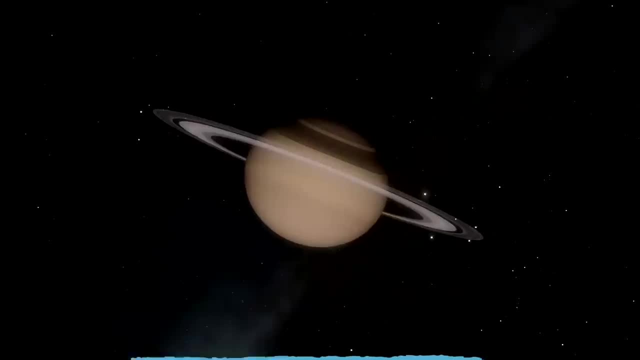 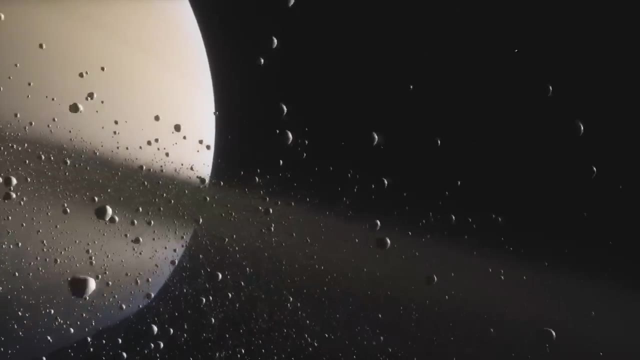 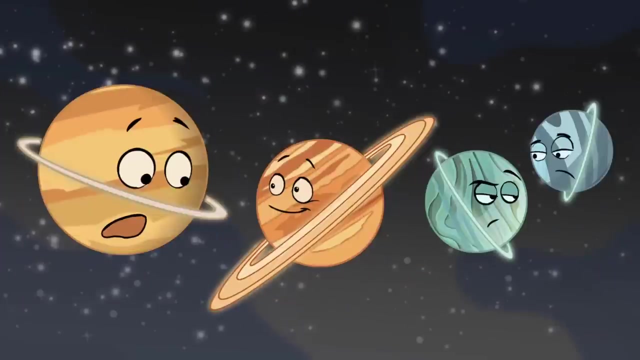 Can you guess how many? Eighty-two? Saturn's strong gravitational pull breaks apart the rocks. Those rocks then spin around the planet, making it look like it has rings. But did you know that Jupiter, Uranus and Neptune also have rings around them? 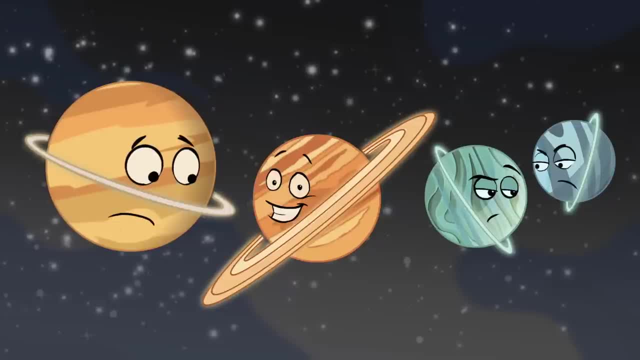 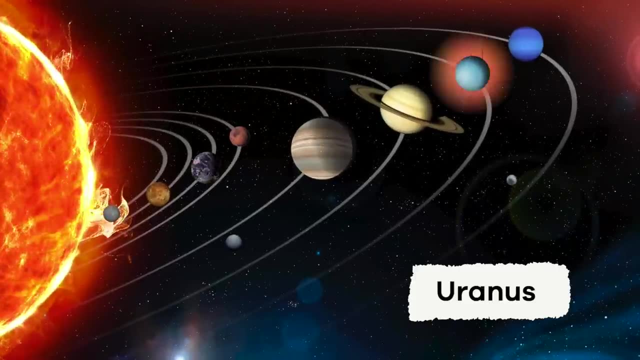 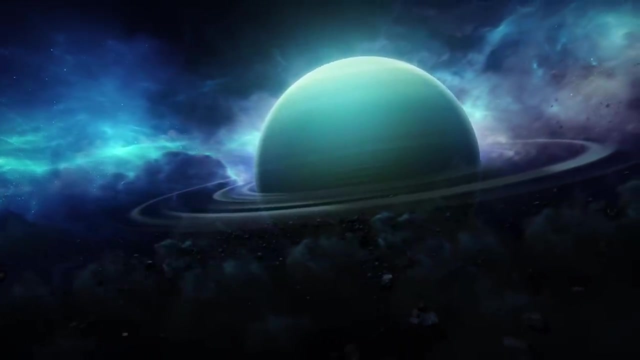 But none of their rings compare to Saturn's Rings and tons of moons. Now, that's a cool planet. Speaking of cool planets, Uranus is known as an ice giant. It is made up of mostly water and it's freezing cold. It is nineteen times farther from the sun than Earth. 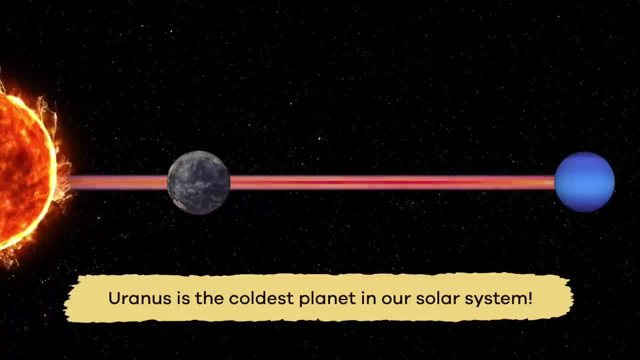 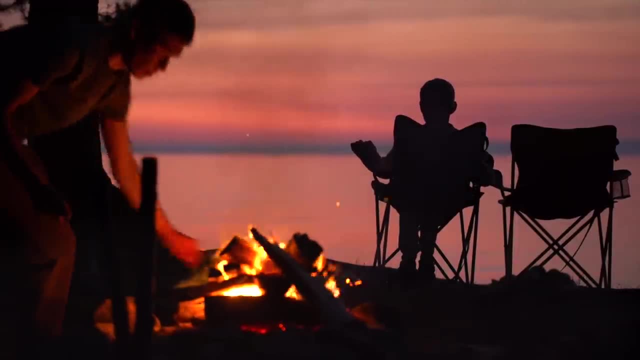 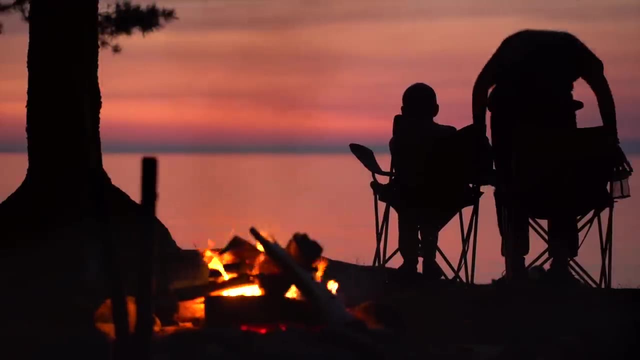 Why do you think that makes Uranus a very cold planet? Well, what happens when you stand by a fireplace to get warm? The closer you are to the fire, the warmer you get right, And the farther away you are, the colder you get. 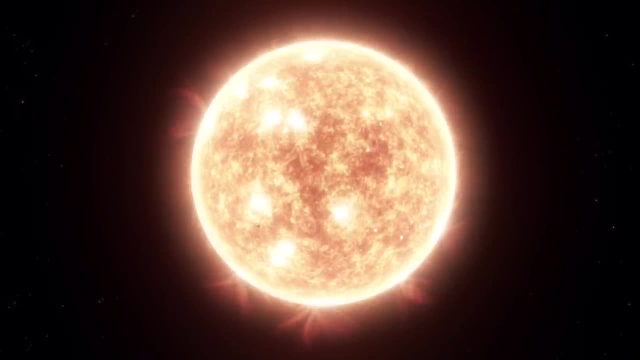 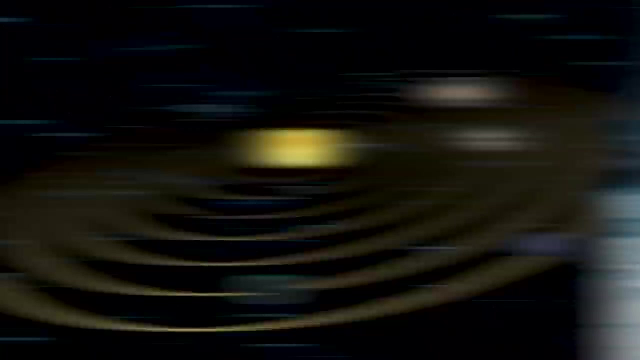 It's the same with the planets in the sun. The planets that are closest to the sun get the hottest And the planets that are farthest away get the coldest, Which explains the freezing cold temperature on Uranus and why people can't live there either. 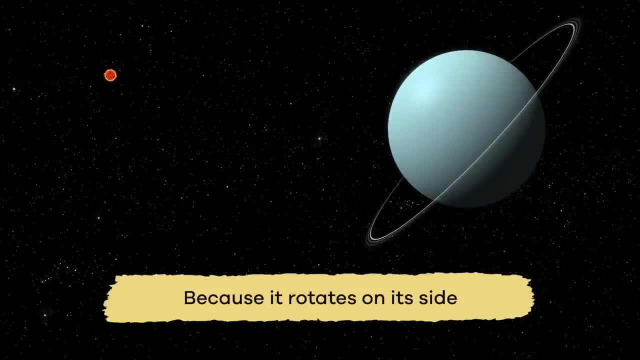 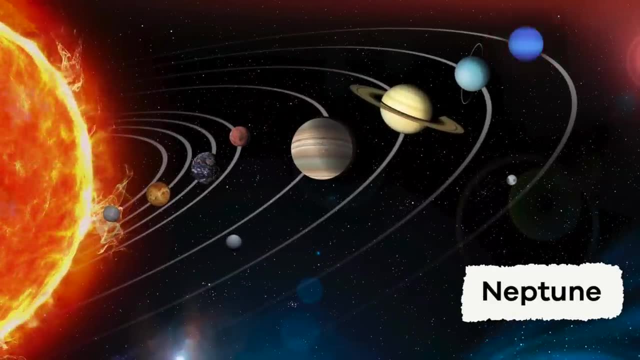 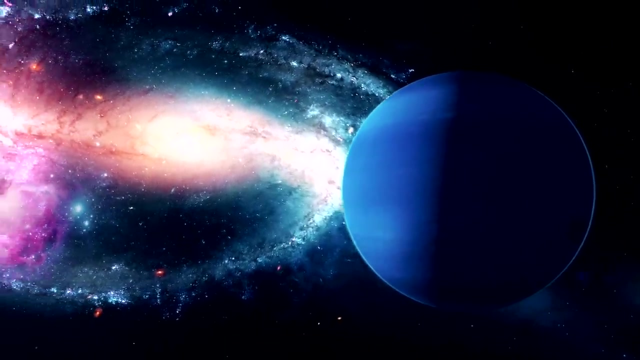 Uranus is also known as the sideways planet because it rotates on its side. Neptune is the farthest planet from the sun. In fact, it is so far away that it is the only planet that we can't see from Earth without a telescope. 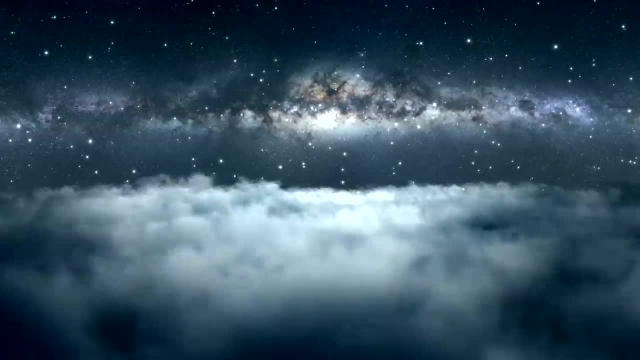 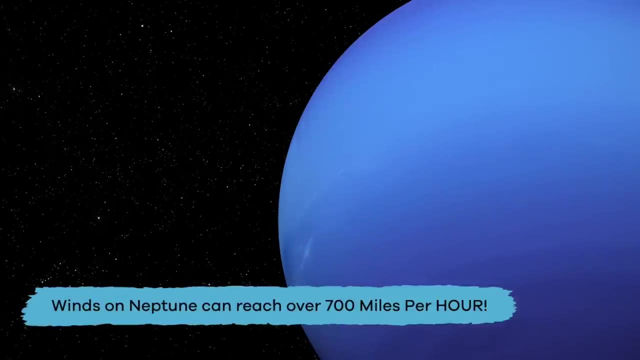 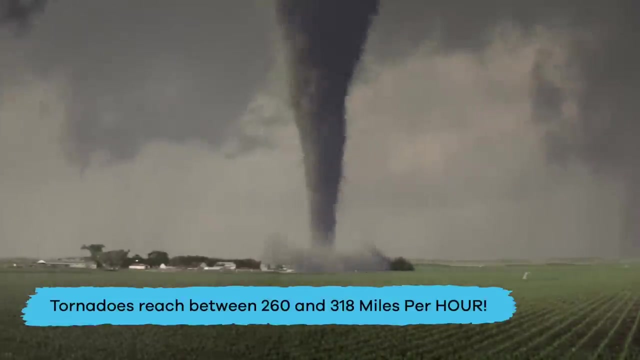 Neptune is dark, cold and very windy. Winds on Neptune can reach over 700 miles per hour. To give you an idea just how fast that is, the biggest tornadoes on Earth can reach speeds of about 260 to 318 miles per hour. 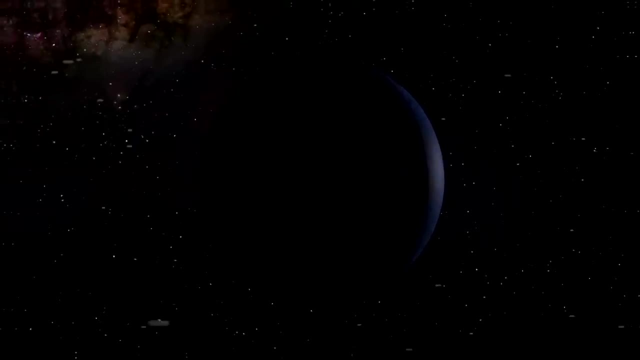 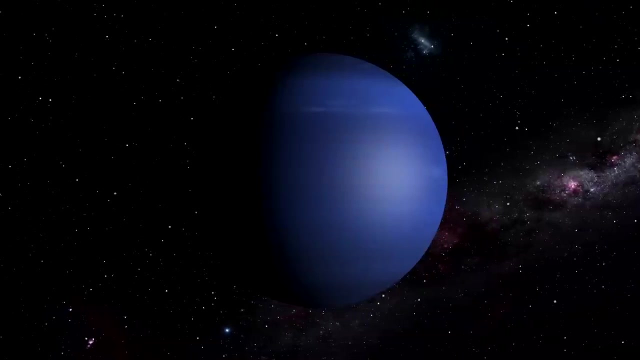 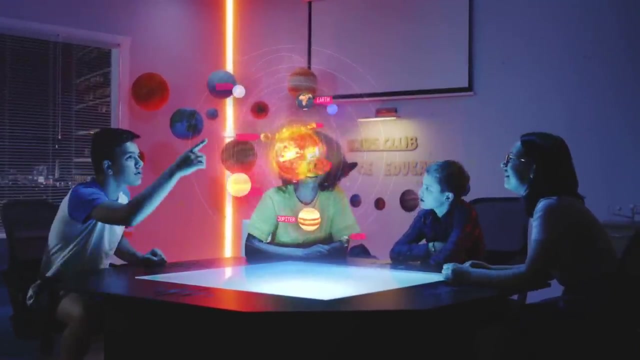 And they can move houses. With crazy fast winds and freezing cold temperatures, Neptune's probably not the place you want to build your summer home. And that's our eight planets. Remembering the names of all eight planets can get kind of tricky. This saying might make it easier. 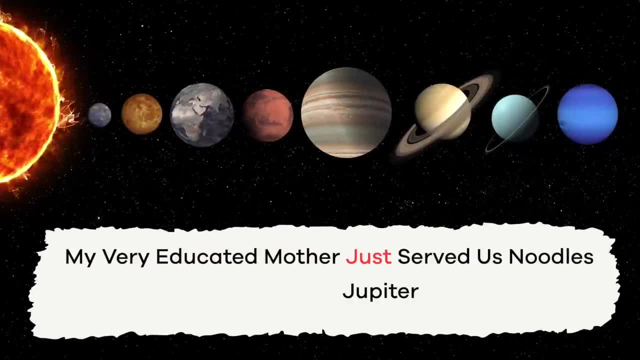 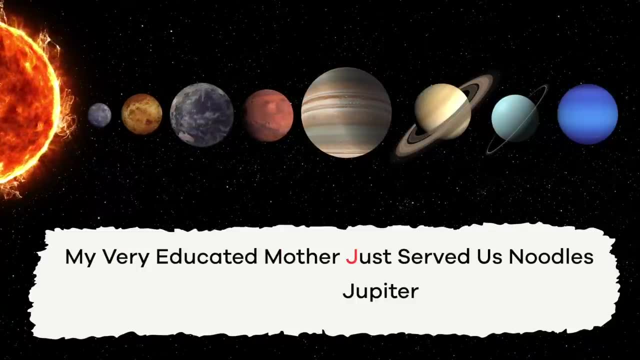 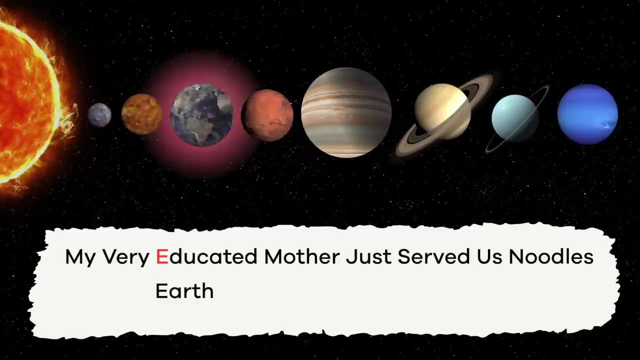 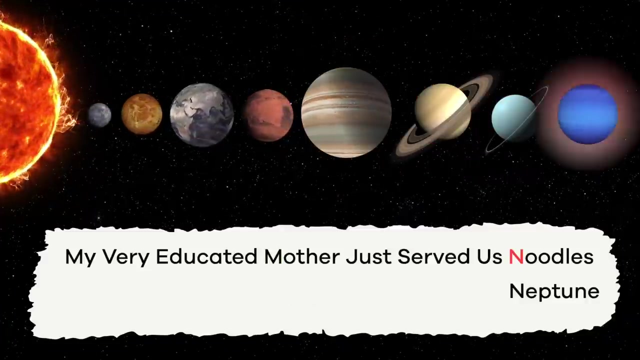 My very educated mother just served us noodles. The beginning letter of each word in this sentence is the same beginning letter as each of the eight planets in order: Mercury, Venus, Earth, Mars, Jupiter, Saturn, Uranus and Neptune. Cool planet fact. 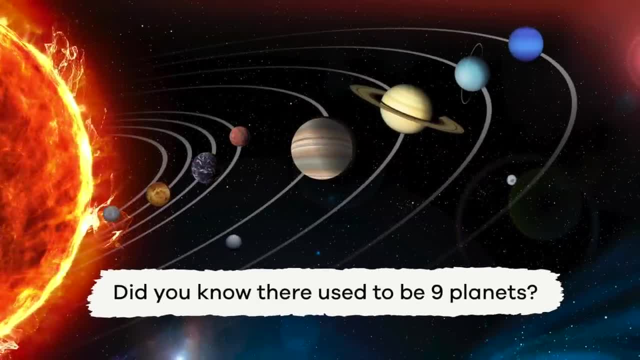 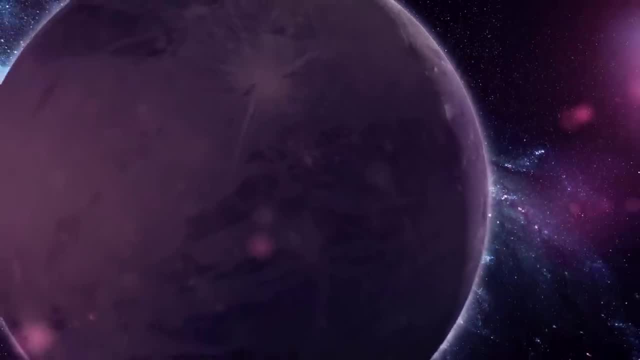 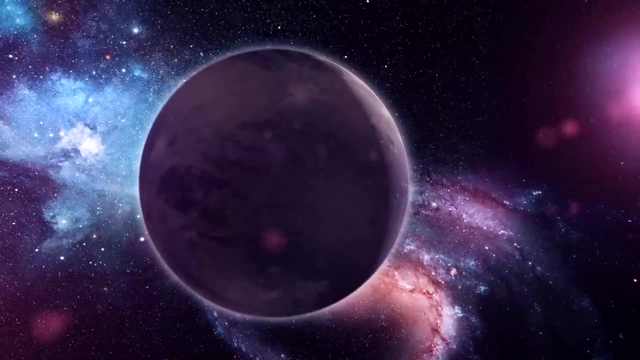 Did you know that there used to be nine planets in the solar system? My baby, Pluto, was the name of that other planet. It didn't disappear, It just got downgraded from a planet to a dwarf planet. Sorry, Pluto, Pluto didn't do something wrong. 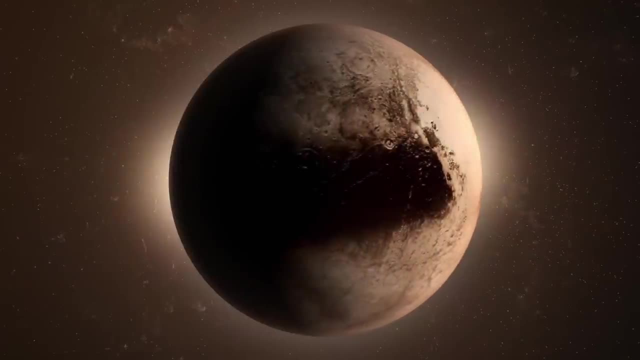 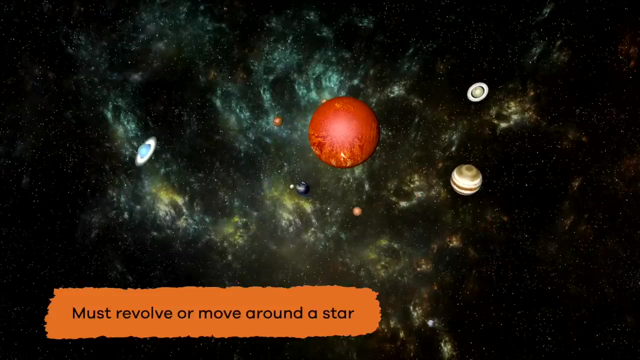 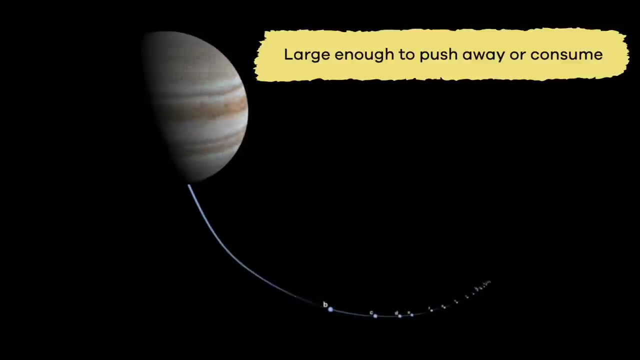 It just didn't meet all the criteria to be called a planet anymore. Remember the three things planets require to be called planets: They must revolve around a star, They have to have enough gravity to be round And they must be big enough to push away. 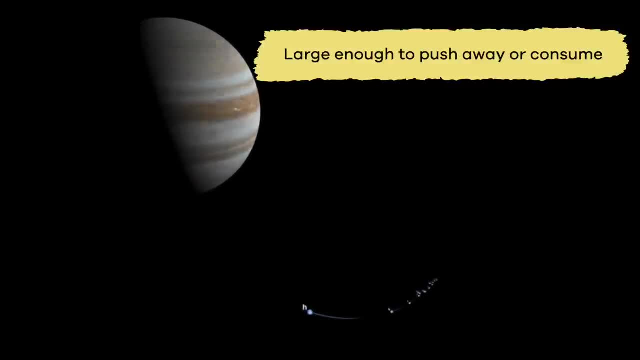 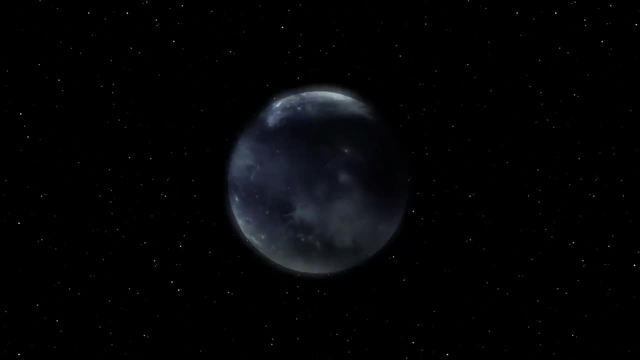 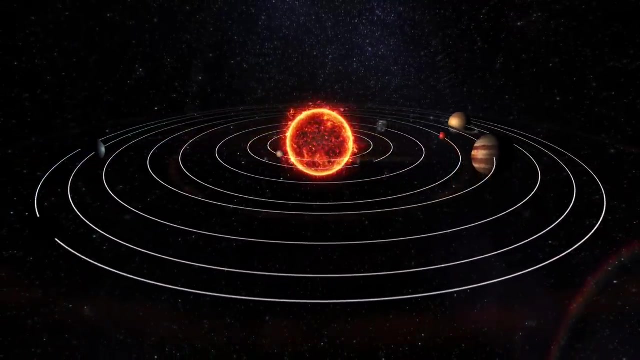 or consume other objects in their path. Pluto got the first two, But it simply isn't big enough to push other big objects away from itself. Now that you're a pro on all the planets, let's pull out our telescope. What planet am I looking at?